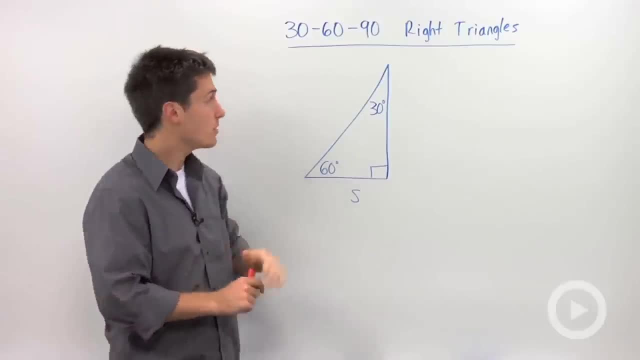 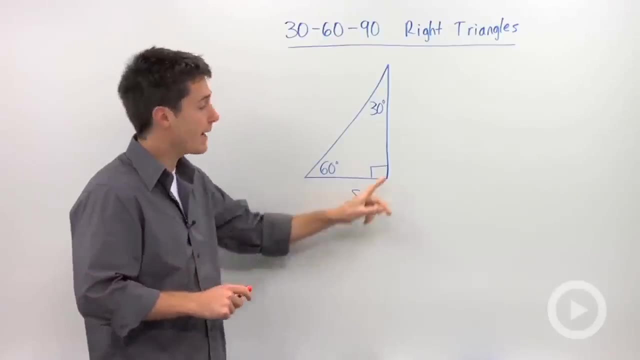 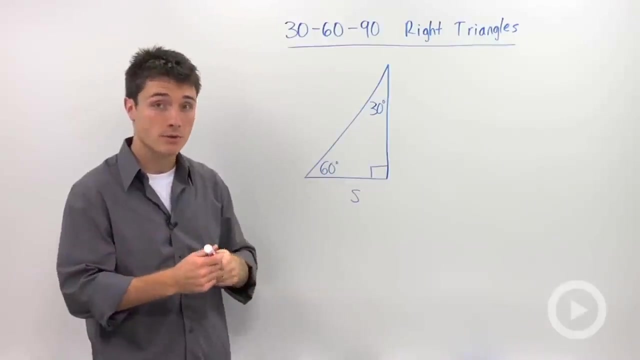 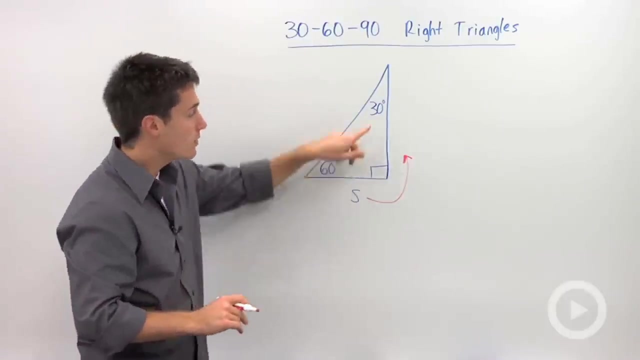 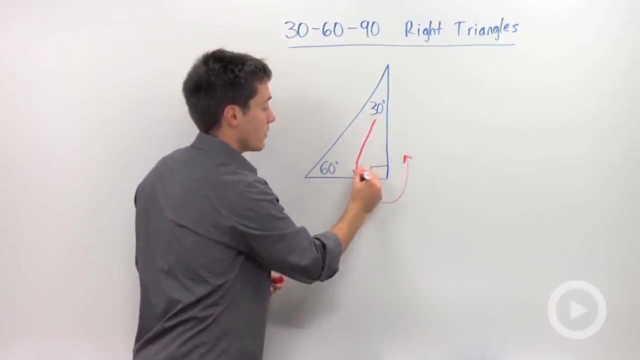 and 30-60-90 triangles. Now what's special about this 30-60-90 triangle is that of the three sides that are all going to be different, I only need to know one and I can find the other two. So that's pretty amazing that of the three sides of a triangle, when it's a 30-degree, a 60-degree, and a 90-degree, I only need to know one side and I can find the other ones. So the shortcut, and again this is based on the Pythagorean Theorem, is to find your longer leg. Now how do I know that this is my longer leg? Well if I look at my angle measures, 30 degrees is my smallest measure, which means the side that is opposite of 30 will be my shortest leg. The next longest will be my next largest angle. And since 60 degrees is smaller than 30 degrees, I can find the other two sides of the triangle. 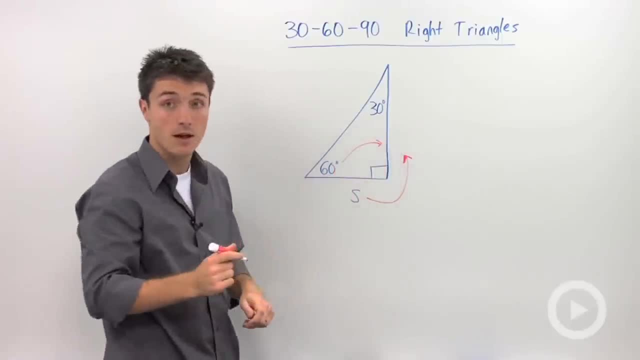 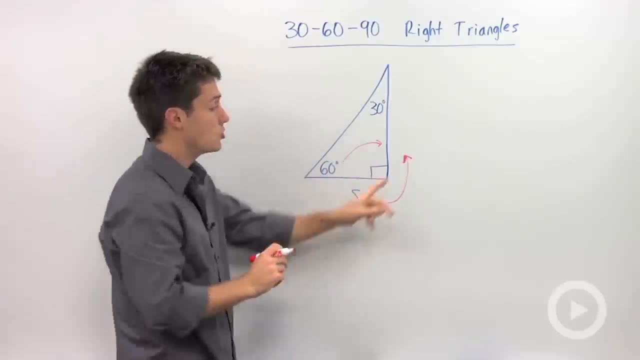 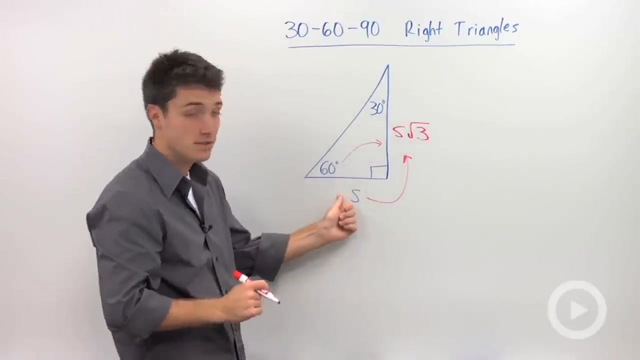 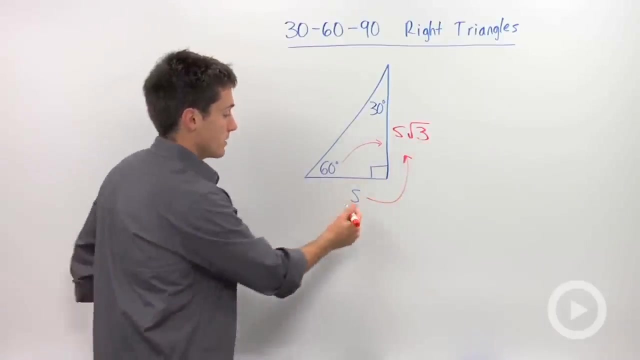 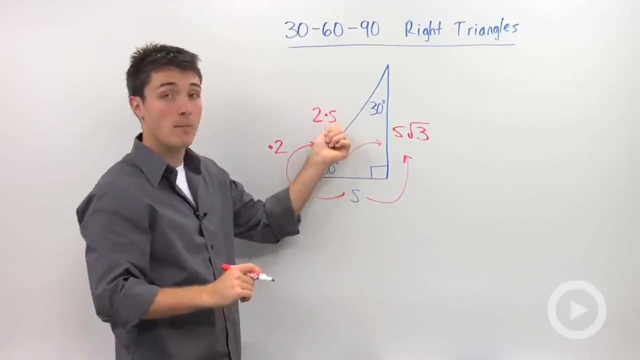 Since 60 degrees is smaller than 90, 60 degrees is my next longest leg. And then of course our hypotenuse is always the longest side in our triangle. So to go from our shorter leg to our longer leg, I need to multiply by the square root of 3. So if this side is let's say 5 units, then your longer leg will be 5 times the square root of 3. Now let's say you want to find your hypotenuse. To go from your shorter leg to your hypotenuse, all you need to do is multiply by 2. So this is going to be 2 times s. So if s is 5, your hypotenuse will be 10. So this works in both directions. So let's say you had your longer 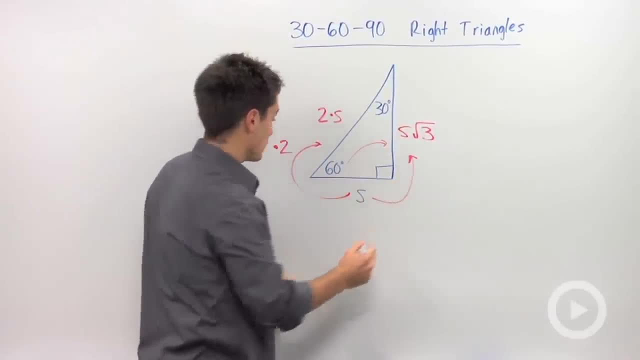 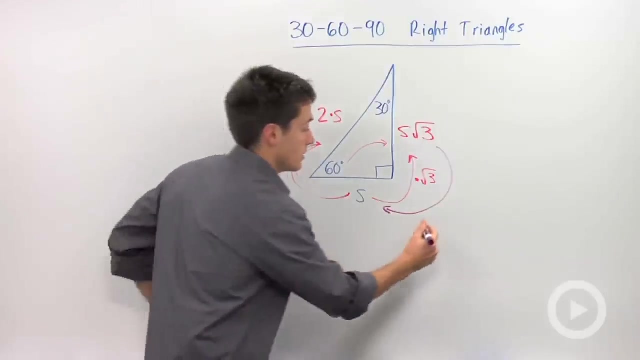 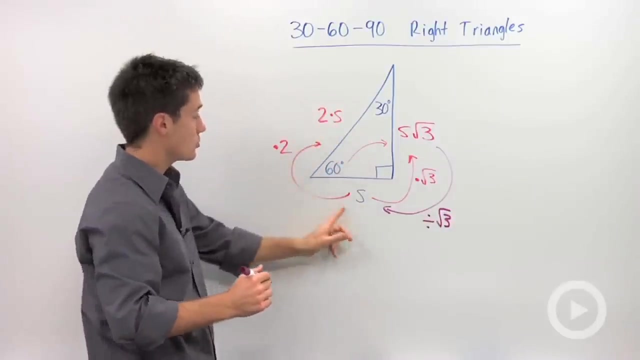 leg and you wanted to find the other two sides. Well first, and actually I guess I forgot to write down right here that you would multiply by the square root of 3. So let's say you wanted to go in the opposite direction. From your longer leg to your shorter leg, you would multiply the squared leg By the square root of 3. Remember to go from your long leg to your shorter leg. Well the inverse operation of multiplying by 3, is to DIVIDE by the squared of 3. The inverse operation of going from your hypotenuse to your shorter leg, is going to be not multiplying by 2, but dividing by 2. So the key leg in this triangle, is this shorter leg. Because from here you can find your hypotenuse, by multiplying by 2. And 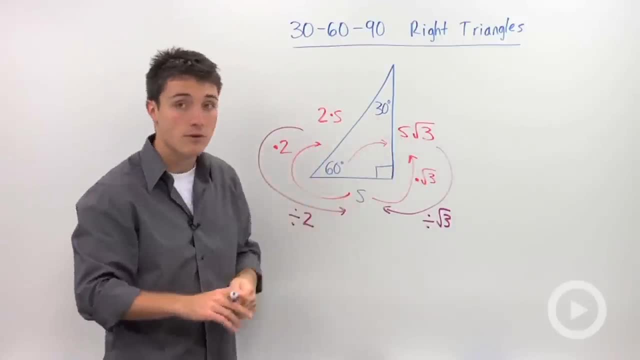 you can find your longer leg. So use these shortcuts whenever you see a triangle with 30, 60, and 67 units you want to have speed to. To apply this to thinchness, you should 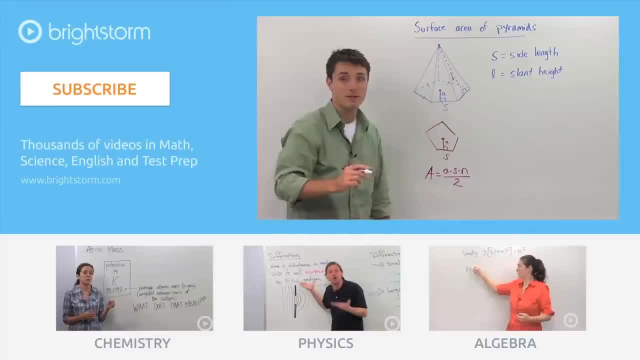 90 degrees and by two I can't do this with you two laughing back there so if